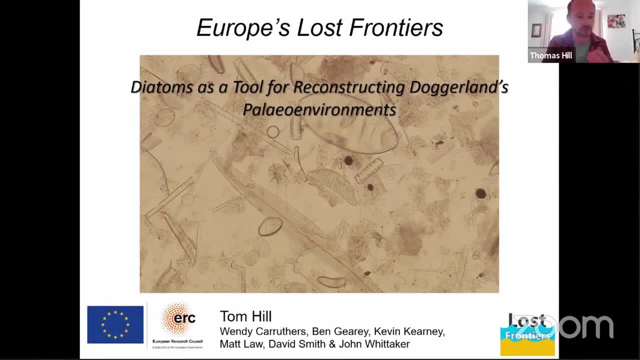 overview of some of the results based on applying diatoms as a tool for reconstructing Doglands paleoenvironments. As highlighted by Ben and by Martin, we are in the early stages of synthesising a lot of this data. I've tried to incorporate some of the results from many of my 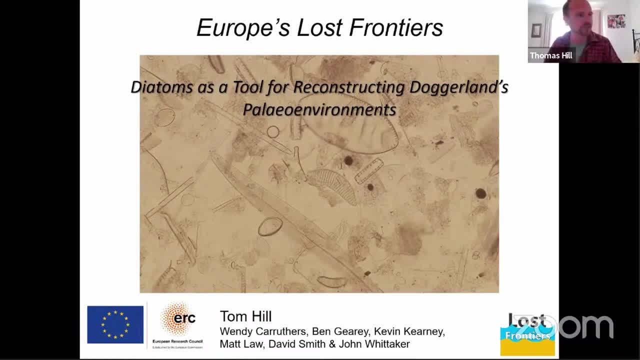 paleoenvironmental colleagues who are accredited at the bottom of this slide. But again, we are looking at provisional data and I also have to put a disclaimer. I apologise in advance. I also have lots of diatom diagrams and I'm nowhere near as good as creating diatom diagrams as Ben is. So 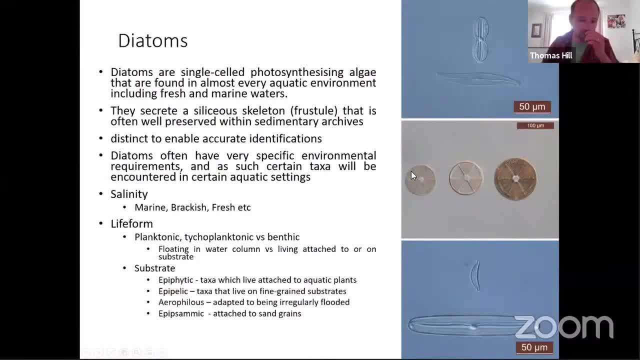 they look a little bit rubbish, But in light of the size of the audience, I wanted to in the first instance highlight, you know, introduce a little bit of the data. So I'm going to start off by showing you a couple of diatoms. Not everybody may be familiar with what the critters 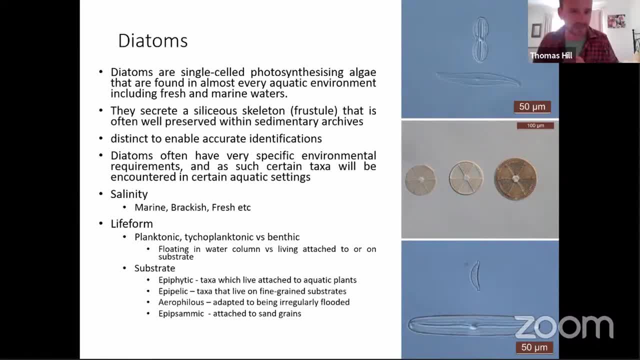 are So? very briefly, these are single-celled photosynthesising algae that are found in almost every aquatic environment, whether you're looking at freshwater lakes or open marine settings. They secrete what's called a frustule, a siliceous skeleton, and it's often very 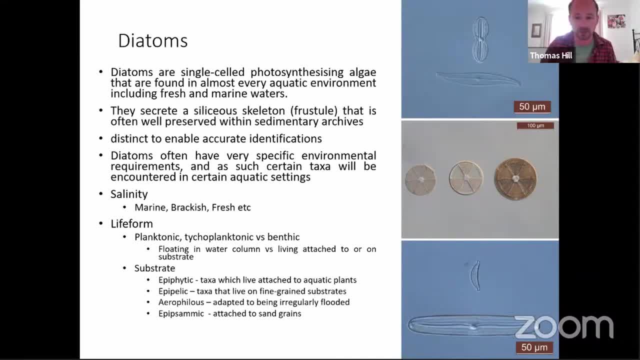 well preserved in sedimentary archives, particularly mineralogenic archives. So these are things like muddy, sandy deposits not as well preserved in peatlands as we'll find out about. They thrive in peatlands, but their preservation is limited over time. 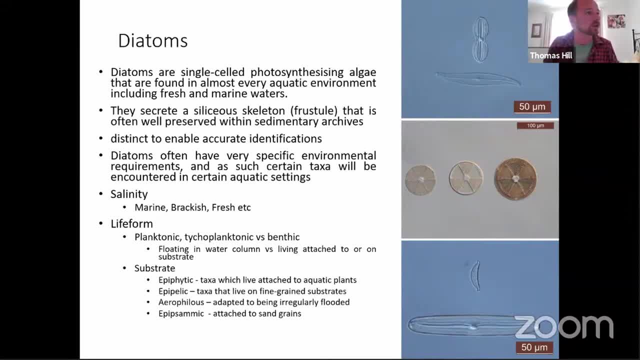 as that peat gets buried. They are also really useful because they're very distinct and you can see a few images on the right of your screen showing the morphological variety in terms of the shape of these little critters, And I think it's also useful to appreciate scale. 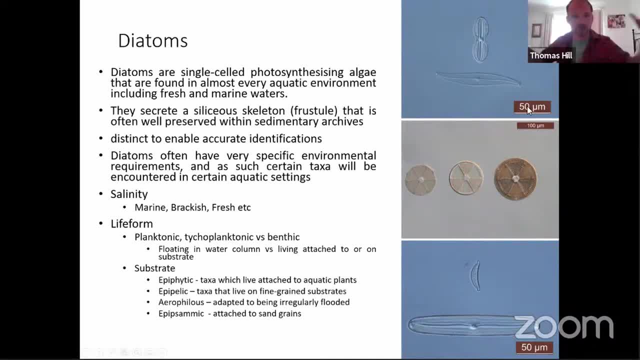 To date we've, you know, especially with Marty's presentation, we were talking about very, very large-scale reconstructions. We're going into the micro now as, similarly with the pollen, with Ben- This is here on the right-hand side- is a genus Actinophicus, a marine plankton. 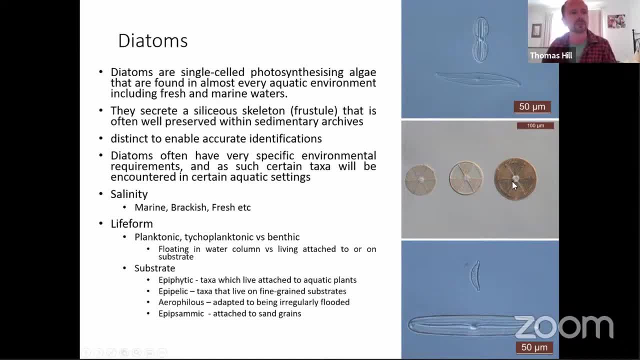 taxa approximately 100 microns in diameter, And so there are a thousand microns in a millimetre. So you line 10 of these little critters up to make up just one millimetre on your ruler on your desk. So very, very small. The great benefit of diatoms is that they have very specific environmental. 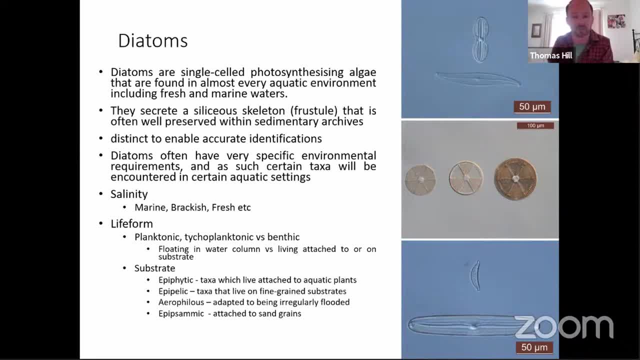 requirements which mean that certain taxa will be encountered in certain aquatic settings, whether that be fresh, brackish or marine. If we looked at salinity as an example, we can go into more detail and I'll allude to this in the presentation because we can talk. 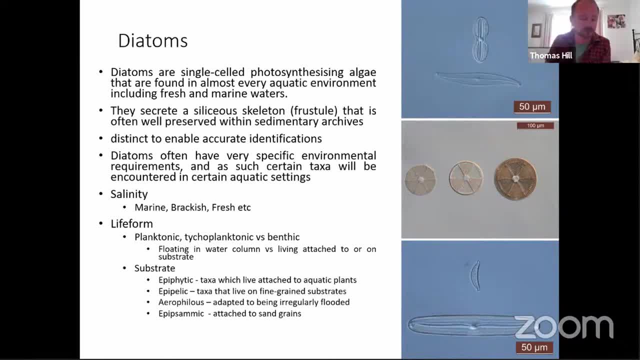 about life form as well. Some taxa live floating within the water. These are planktonic taxa. Others live attached to or within the substrates underlying the water, which these are the benthics, And we also get a bizarre group called the Tychoplanktonic taxa that sometimes are associated. 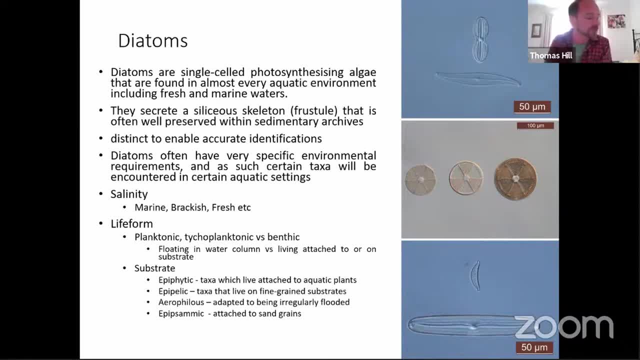 with living on the substrate, but can also be found floating in the water column. Now we can then go into further detail, especially with the benthic taxa. So these are the ones attached to or living on the substrates, because different species prefer different types of 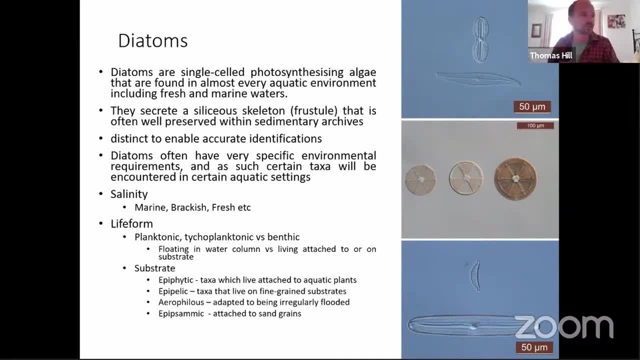 substrates. There are taxa associated with aquatic plants such as epiphytes, which are called the epiphytes. We have epipelic taxa. These are the little critters who like being attached to or living on muds, very, very fine grained sediments. 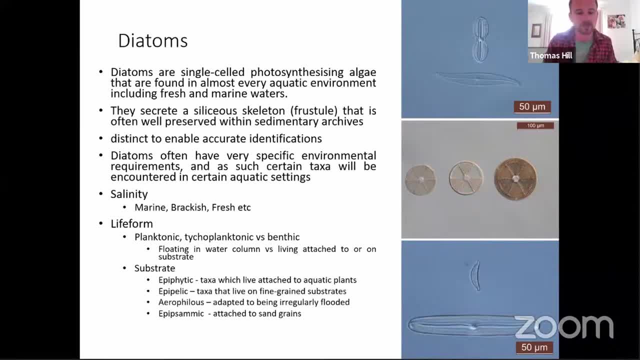 there are also aerophilus taxa, And these are taxa that are adapted to being irregularly flooded, So that could be on the margins of a lake or, more often than not, in the intertidal zone, if we're looking in coastal settings. And then there are epipsamic taxa. those often 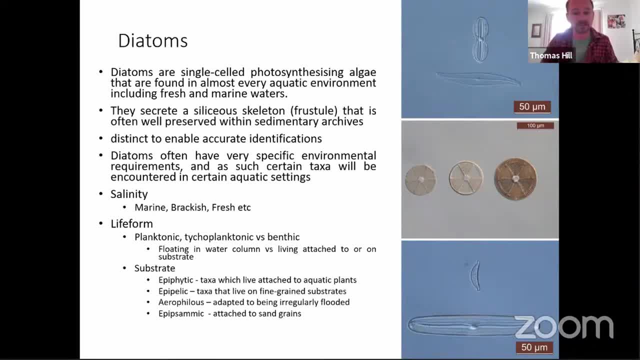 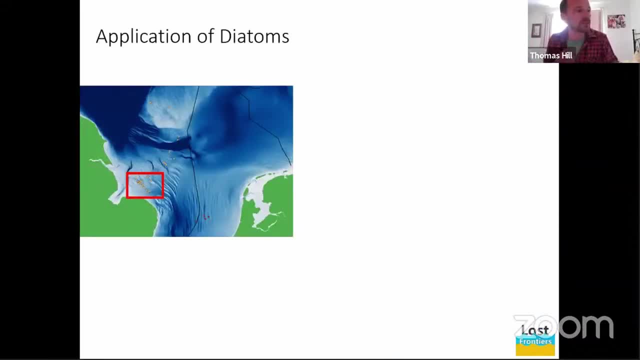 attached to sand grains, which are more common in things like riverine settings. So we've seen this diagram quite a few times already in terms of the location of many of these cores that were extracted as part of this diagram. So we've seen this diagram quite a few. 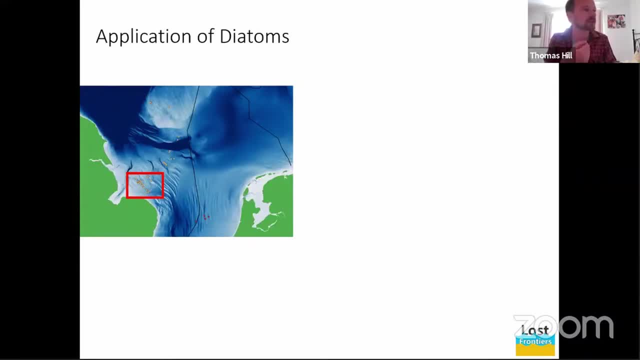 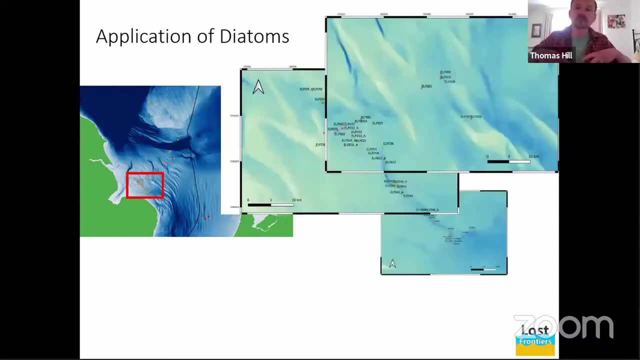 times already in terms of the location of many of these cores that were extracted as part of the the project, and we are going to be. I'm going to be focusing on a selection of cores within this area- Ben alluded to as well- And I'm going to try and provide a generalised 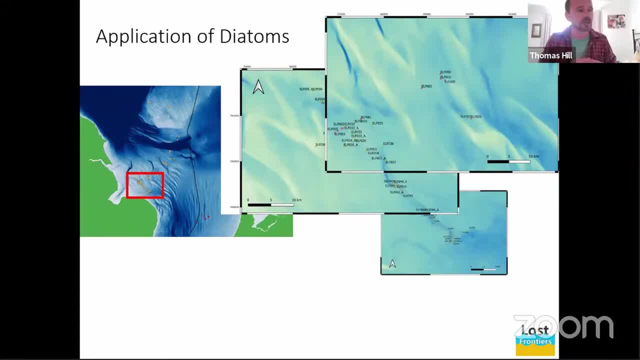 summary of the results. There's been a lot of analysis that's been undertaken, But I'm just going to broadly divide them into two groups. First I'm going to explain two cores that have been identified as having late glacial freshwater depositional sequences. 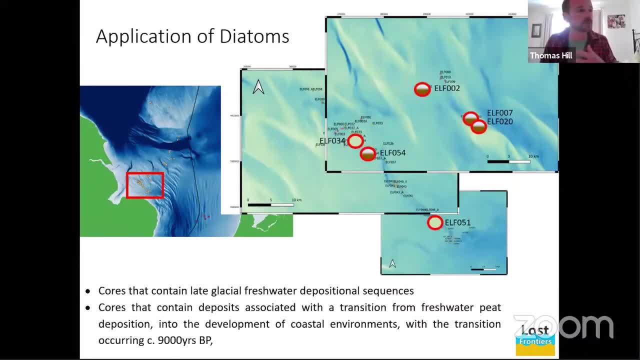 And then I'm going to talk a little bit about some of the cores that have very valuable sequences, that show a transition from peaked deposition into the development of more established coastal environments, with the transition appearing to be relatively uniform across the area of around about 9,000 years BP. And considering the aim of this project is to 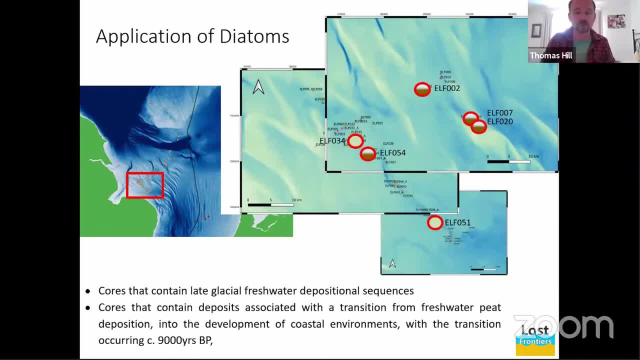 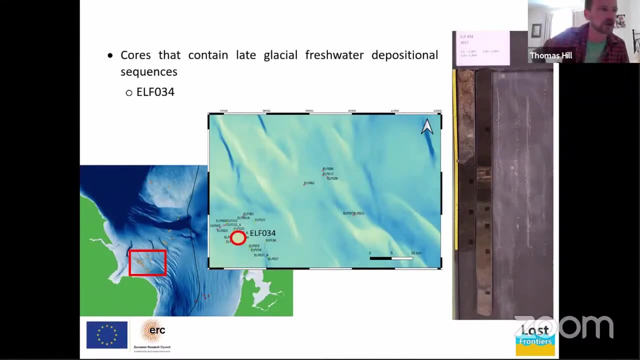 understand Doggerlands and its eventual loss to the advancing seas. it's a really important part of this project as well. So if we were to start off with basically a walk-through time, we're going to start with the oldest sequence that I have encountered, which contains diatoms. 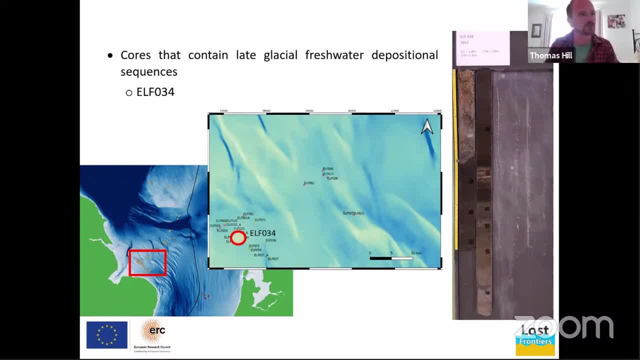 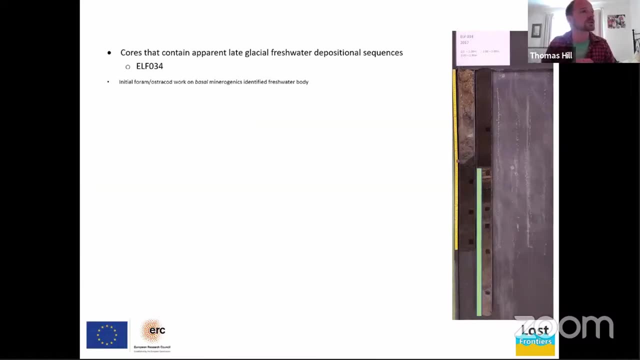 and indeed contains other lovely little things to contribute to our understanding of the late glacial period within Doggerlands. And Ben, and indeed Martin, alluded to L34, and Ben indeed commented on the one section of the sequence. So one thing that I would like to acknowledge is the outstanding work done by John Whittaker. 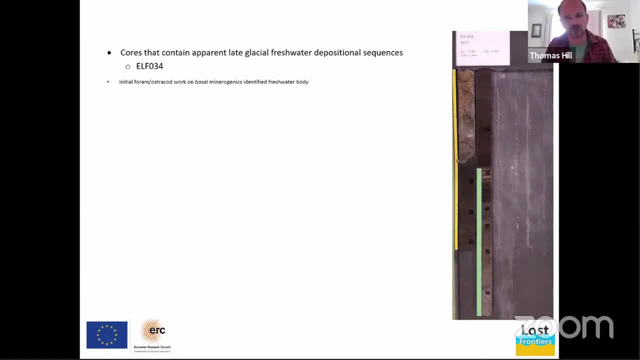 who, again Martin highlighted, did a rapid assessment of every single core to give us an approximate understanding of the overall water conditions that prevailed for many of these sequences. And John encountered, through his initial ostracon and foram work, that the basal section of this core was full of fresh water forams and fresh water ostracods. 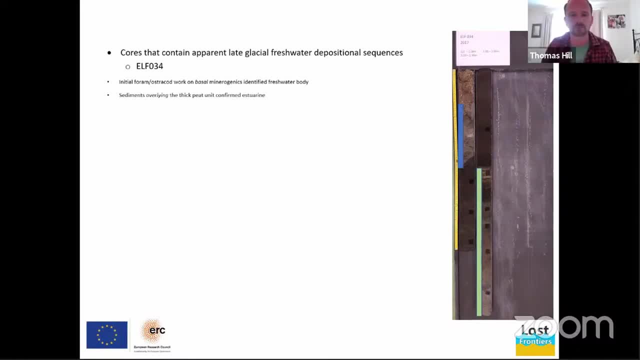 So he also found an abundance of open or estrine taxa within the overlying immunogenics, And in between we have this relatively thick, one metre peak units which we are now finding a lot of information about as this project progresses, And indeed 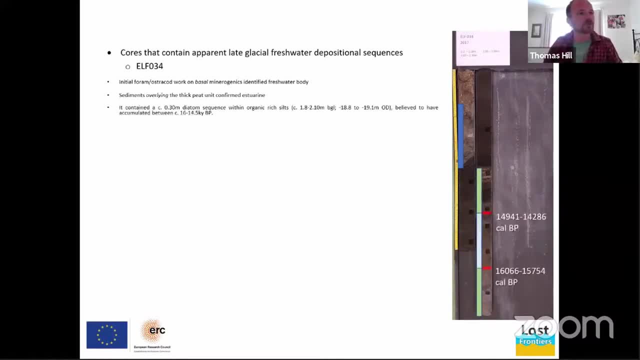 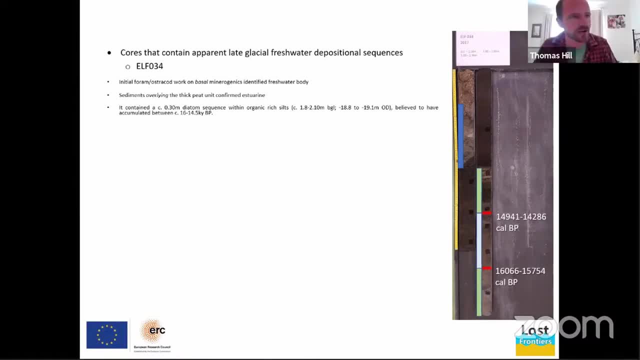 They were non-oxidant, They were non-oxidant, They were non-oxidant, And radiocarbon dating provides us with a relatively reliable signal. Now, this is bearing in mind that Ben's talk was predominantly on the upper section, going into the peat. I'm 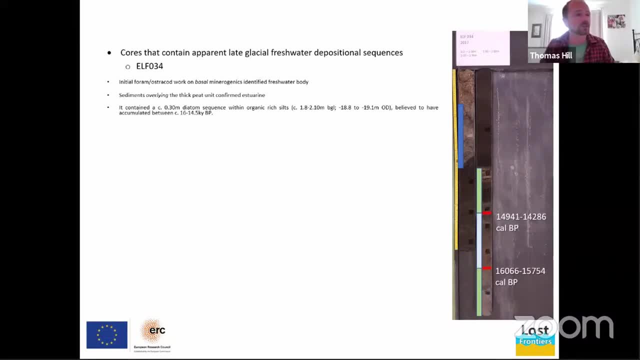 looking a little bit earlier so we've got slightly older dates, But at least for the section of the core in which diatoms were present, we can be confident that this accumulated between approximately 16,000 and 14,500 calbp And, if accurate, this place, if accurate. 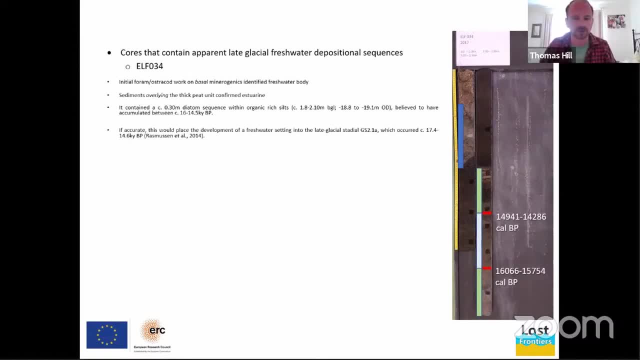 this places this period of freshwater deposition into the late glacial stadial, which occurred between 17 and a half to 14 and a half, and for those to give context for those individuals who may not be familiar with this, we are looking at the very cold period prior to the onset of 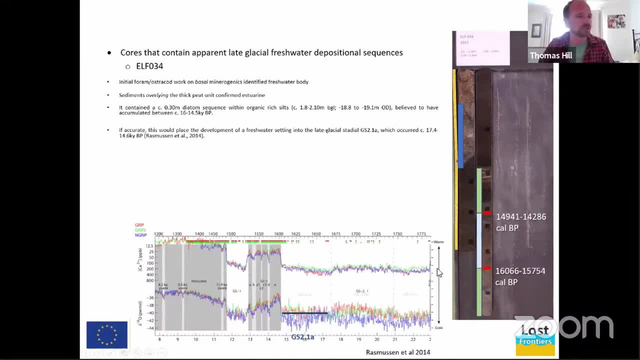 climatic warming. this is just one of the Greenland ice cores and it shows temperature essentially through the oxygen isotope record. so this whole thing here is cold, and then we go into these warmer periods subsequently, but the diatom record seems to be focused only on this late. 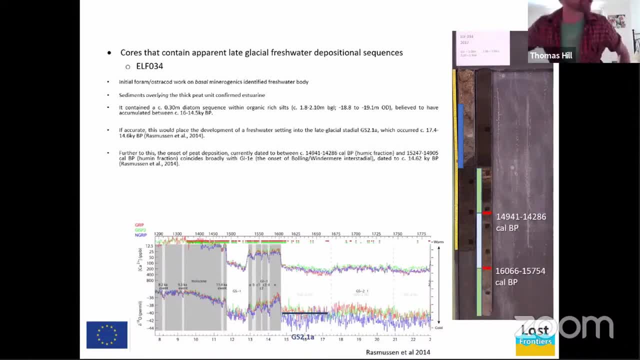 glacial stadial episode and the onset of peat deposition is currently dated to between or to around about 14 and a half thousand, and again some modelling needs to be undertaken on this to give us secure understanding. but we're confident with the dates. but this would suggest that the peat 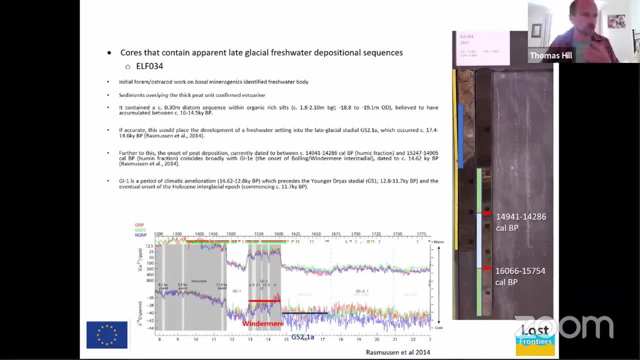 deposition, then it becomes initiated during the windermere- or bonning, depending on which term you want to use, or gi1, which then suggests that within the peat that overlies it, we also have the potential to preserve the Younger Dryas and also the Holocene, and this is reinforced by the fact that we have a date. 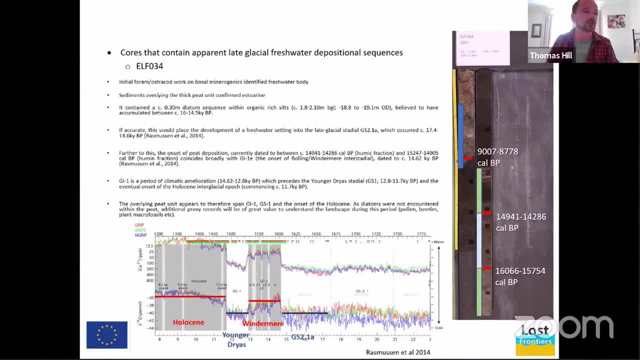 of the peat into estrine deposition around about 9 000 years bp. so we have a meter sequence that has the potential to span quite a considerable period of Earth's history, a quite important period of Earth's history considering the retreat of ice sheets and indeed our understanding of Doggerland. 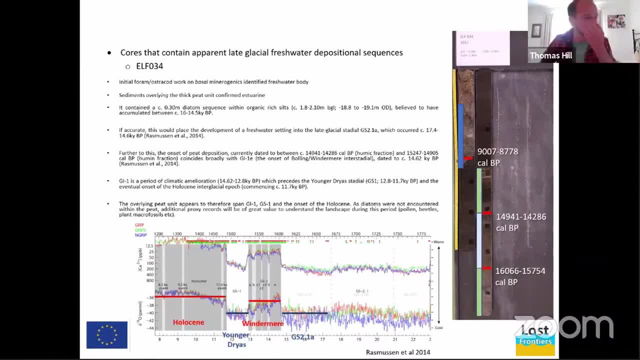 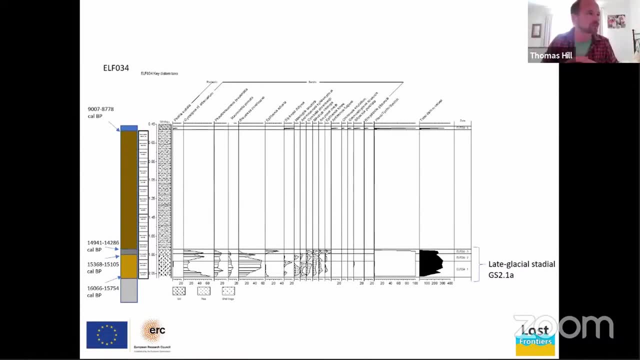 as we move through the late glacial into the early Holocene. So this is a one of the lovely diagrams that I'm sure you're going to detest, primarily because they're so small and it makes it very difficult to read half of the little names on them. but, as Ben highlighted, it's looking at a 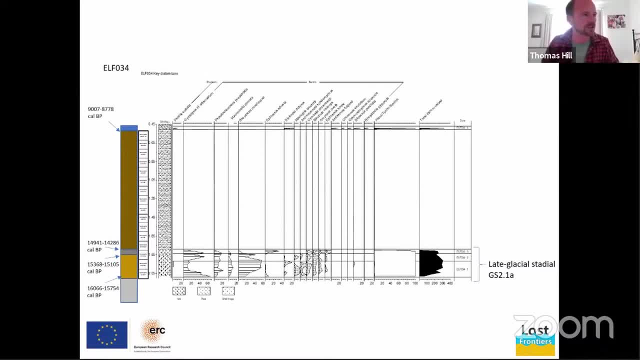 vertical profile food sedimentary sequence. I've highlighted a couple of the key. radiocarbon dates and indeed diatoms are restricted to the basal section prior to peat deposition. but just to stress that we're looking at here now we've got this. all the work is ongoing. due to the delays as 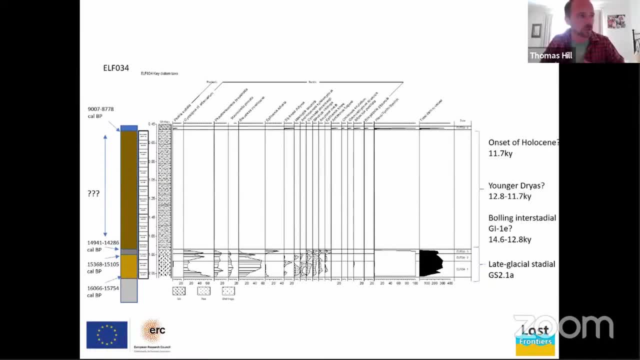 we're all familiar with, but we have a potential to have a sequence that could- a peat sequence in fact. you know, this is an organic sequence that could shift through the entire late glacial into the early Holocene, and it's reinforced by the fact that some of the work that Daggett Smith's 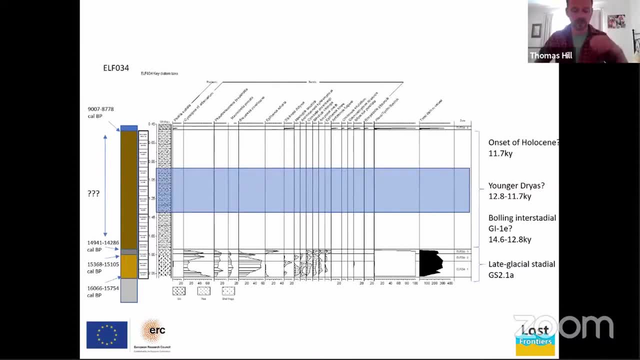 highlighted, has identified a small but suitably interesting beetle signal within a number of the pools that were taken that indicate cold climate. so we are relatively confident that we have a conformable sequence and indeed the radiocarbon dates also show conformity throughout. so it's going to be really interesting to hear this develop over the coming months and indeed next. 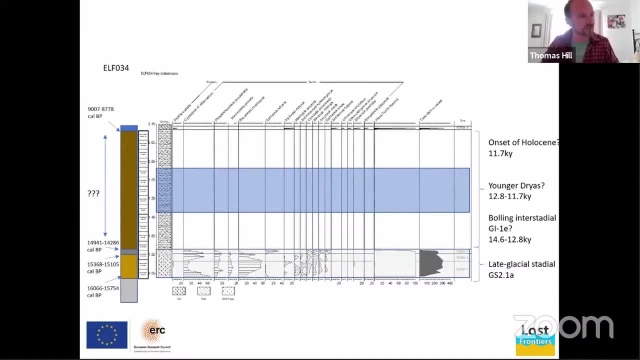 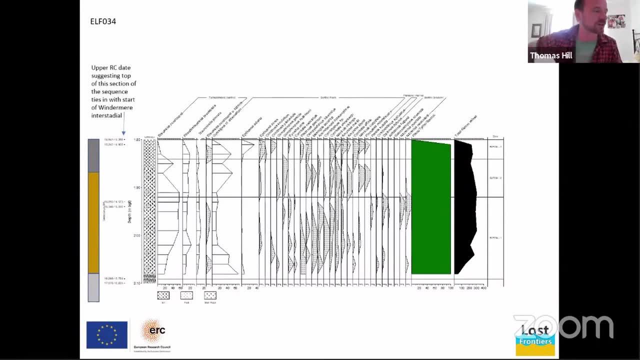 year. so we're going to focus just on this joyous signal down here with some provisional results. yes, trying to explain a single diagram like this in 20 minutes is difficult enough, and I'm trying to get going to get through three or four of them. so again, we 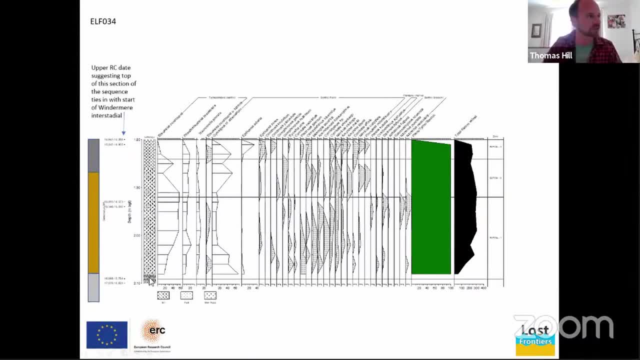 highlight the radiocarbon dates. we're looking at the low most section, about 0.3 meters. the uppermost date infers that we're looking at around about the onset of the Windermere in stadial here and the radiocarbon dates allude to this being in the Greenland stadial prior to warming. we have. 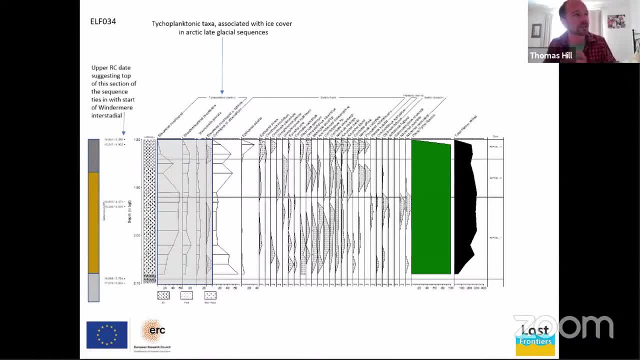 a relative abundance of what are known as these Tycho planktonic taxa and through much research, these taxa are often associated with ice cover in arctic late late glacial sequences. it's reinforced by the fact that there are almost there are no planktonic taxa, and I'll talk about that. 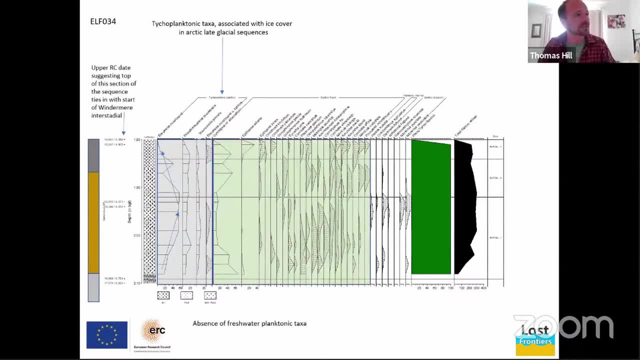 shortly. there's no planktonic freshwater taxa. the, the subordinate grouping are the, the benthic taxa and, as highlighted with these little arrows, there is an increase in the Tycho plankton, then a decrease through this zone and the benthic taxa, specifically this little critter, gyro Sigma attenuatum, decreases, then increases mirroring. 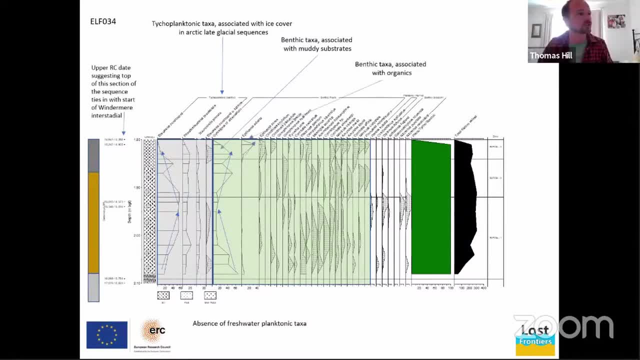 the increase and decrease in Tycho plankton and towards the top of the signal, we have this increase in some benthic taxa associated with organic fragments and organic remains. what's really bizarre is the fact that there is a small but sufficiently significant signal of marine. 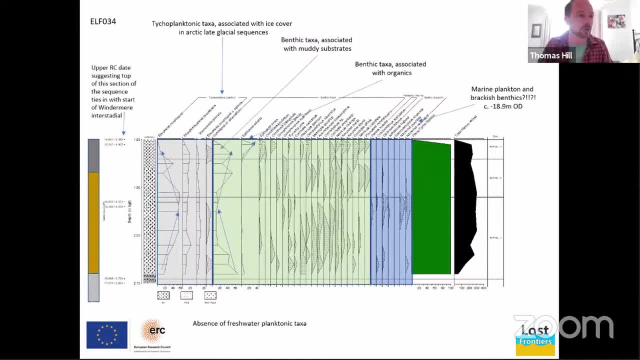 plankton and brackish benthics. um. I also want to highlight some of the other work. you know Ben's alluded to the abundance of pollen, Juniper, you know. then there's these, these aquatic taxa. they're watermilfoil and bullrush, some. 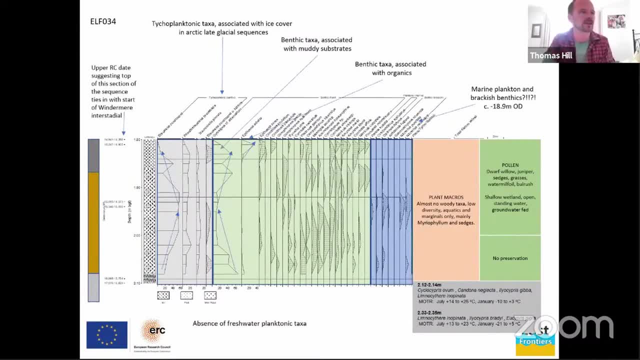 reflection in the plant macros within this section as well, primarily aquatics and marginals. and of greatest interest- and this is how proxy work or proxy analyses always work- there is a relative abundance of ostracods in the section beneath, where my diatoms are encountered and the 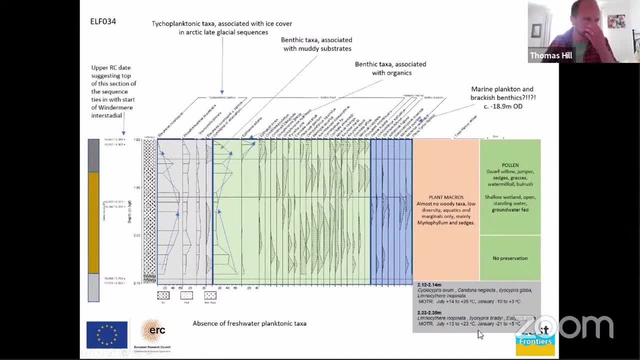 lowermost sample has um, some, um. David Horn has done some mutual climate temperature instructions to infer that the lowermost sample could have winter temperatures of minus 21.. and slightly higher up again, just below my section, winter temple temperatures are still cold, not as cold, but minus tense. we have very, very cold climatic conditions immediately preceding the 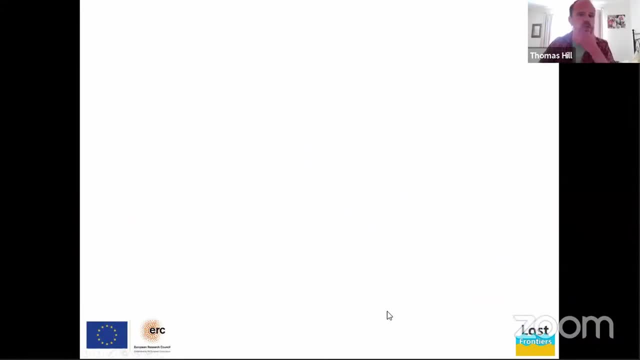 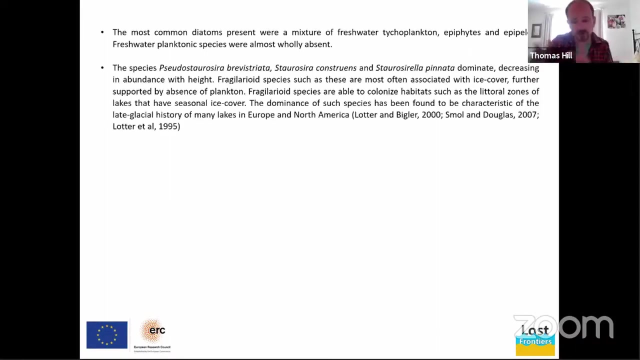 section in which diatoms are in health. um. so, in summary, the most, uh, most common diatoms present are a mixture of these Tycho plankton with a smaller amount of epiphytonic pellon. there are no freshwater plankton species now. the majority of the tycho planktonic taxa known as in a group. 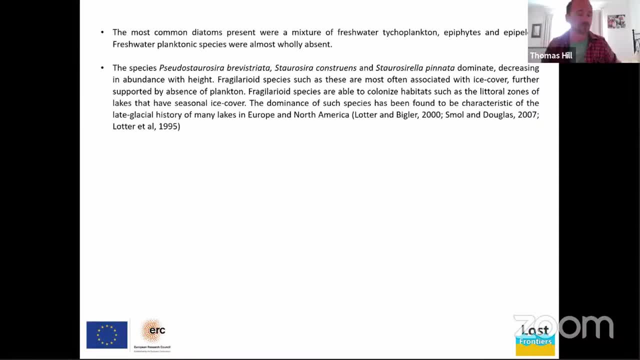 of fragile arioids are most often associated with ice cover, and that's supported further by the presence or the absence of plankton, and these fragile species are able to colonize habitats such as the littoral zones of lakes that have seasonalized cover. we're not talking about permanent. 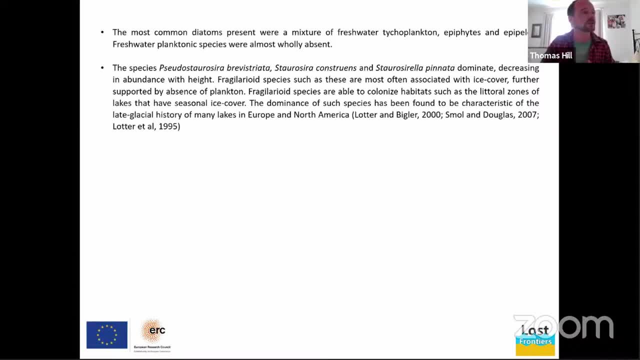 ice cover? I don't think, because we have all these plants in the in the close proximity. that's being, species has been found to be characteristics of many late glacial sequences in northern Europe. We then have these shifts between Fragilarioid species and other benthics, which are likely a 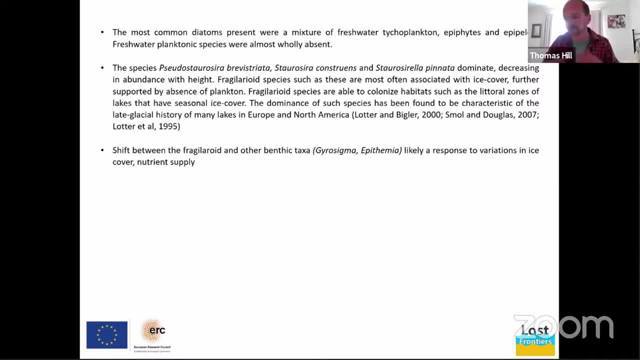 response to the variations in ice cover, seasonality of ice cover and then, which in turn affects nutrient supply and the openness of the water around these margins. And then we have the climatic amelioration due to the onset of the Windermere. 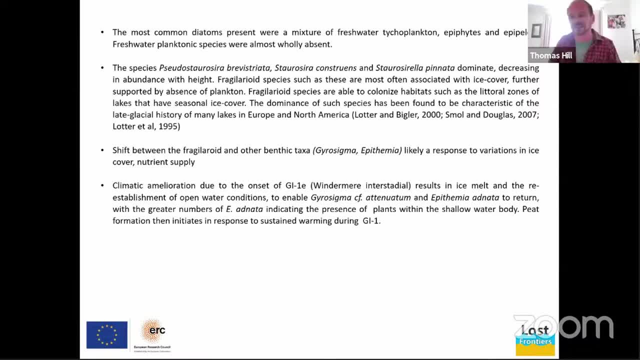 would result in ice melt and the re-establishment of open water conditions and enabling these other benthic taxa to become more typical, and especially the abundance of epithemias, these epiphytes that are more often associated with plants immediately prior to the onset of. 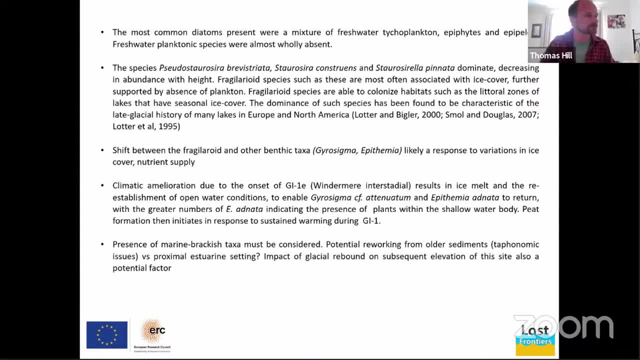 the Windermere, in the stadia or during the transition. The presence of a marine brackish taxa must be considered and I think the most likelihood is that we have a taphonomic issue here. we have reworking of older sediments, If we take 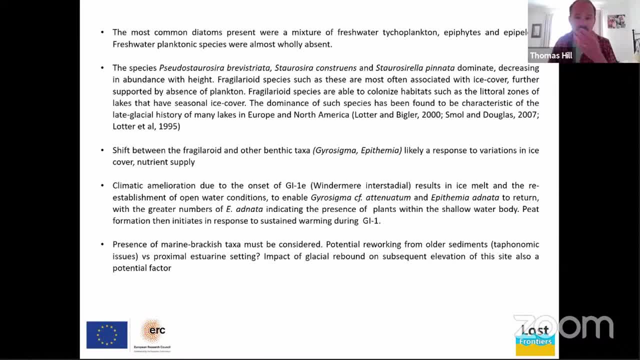 into account the elevation and the likely position of mean sea level 16,000 years ago. we are some considerable distance away from the likely coastline. However, as Martin has alluded to, we are still as of yet fully able to understand the extent of crustal movements. 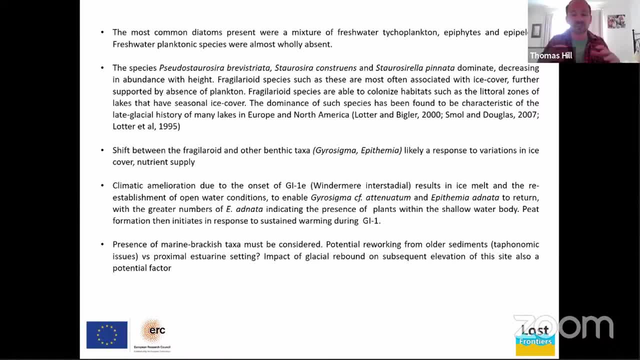 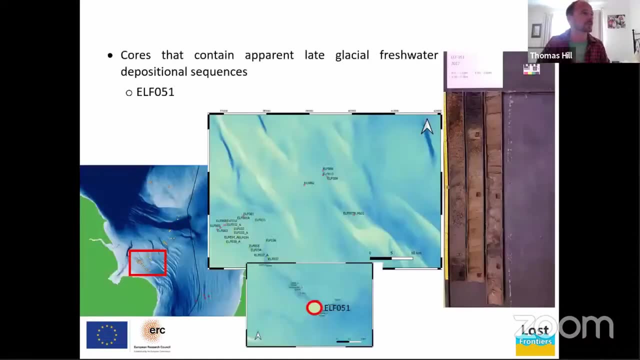 glacier-wise static rebounds and understanding the more localised geomorphological variations to fully discount other factors. But it's very likely that we will have pre-existing earlier sediments that could have been reworked to provide this small but consistent signal. Deep breath, moving quickly on. 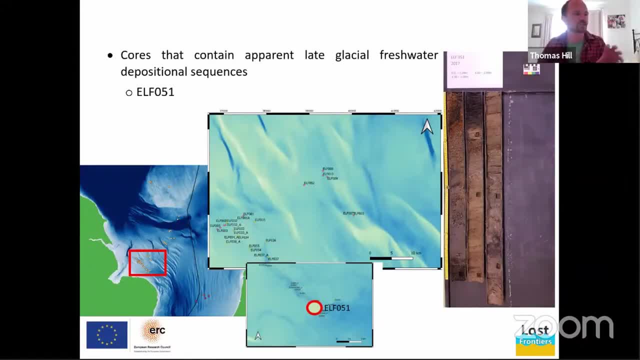 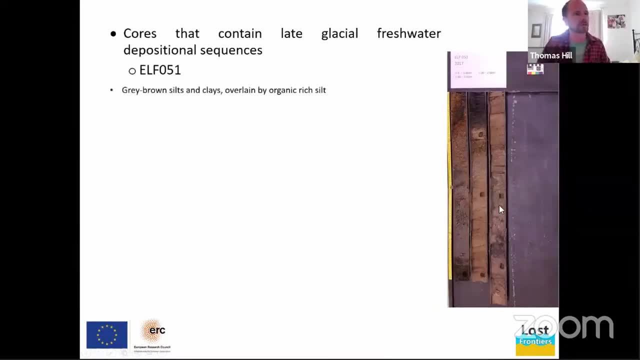 ELF 51 is located at the southernmost section of this southern valley. that Martin provided a summary of Slightly different stratigraphy dominated by mineralogenics, with an organic rich silt rather than a peat unit. And again, fantastic work by John Whittaker. I highlighted 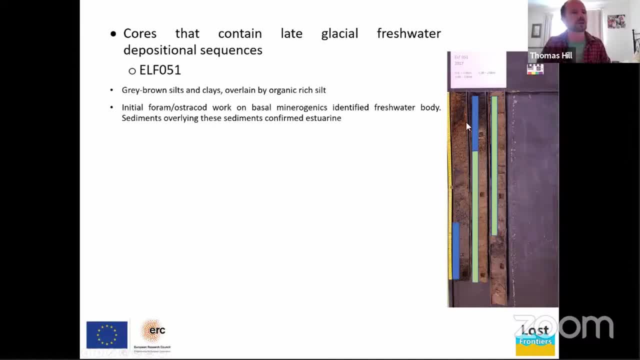 the initial abundance of freshwater conditions which were then replaced by estuarine conditions, which includes this organic silt section, And diatoms were found in abundance throughout the whole two metres. The lack of organic material prohibited radiocarbon dates throughout the sequence and one of the activities we will be doing is working with the OSL results in the 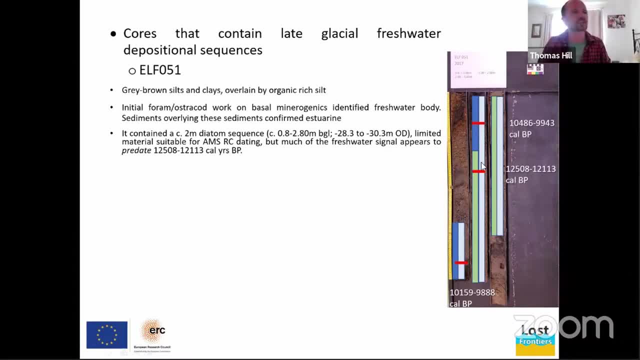 longer term from the underlying strata, But one of the dates from towards the top of the stratigraphy, the freshwater signal identifies that we are looking at around about 12 and a half thousand and from which you could assume, assuming you know, no considerable unconformities. 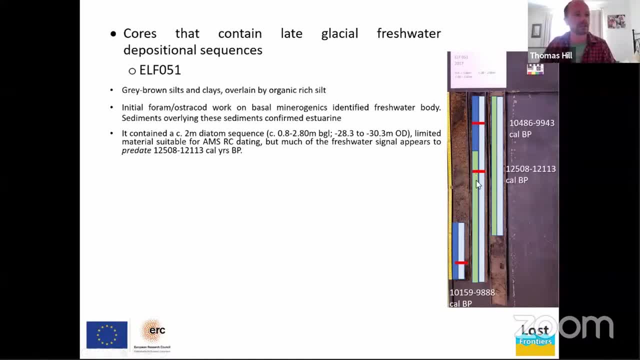 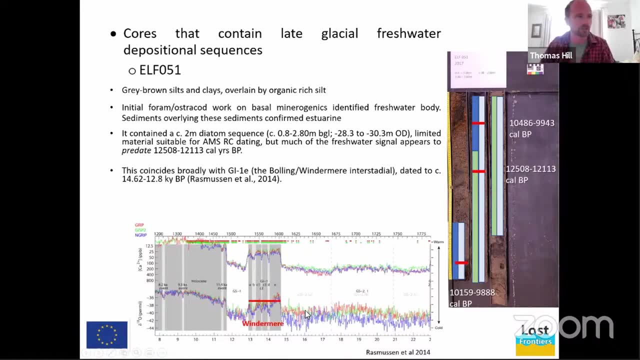 that this material beneath that date is going to predate 12 and a half, and that would therefore put us likely in the windermere, this slightly warmer period. Previously we were looking at the Greenland Stadio, Now we're looking at this slightly warmer, much warmer period. 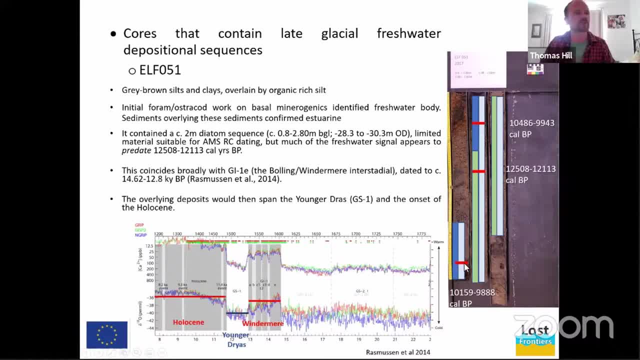 period and again, because of the fact that we have radiocarbon dates towards the top of the sequence that allude to late Holocene, we can have the potential that we could have a section that cut spans the Younger Gerias as well as the earlier Holocene. Another beautiful diagram. 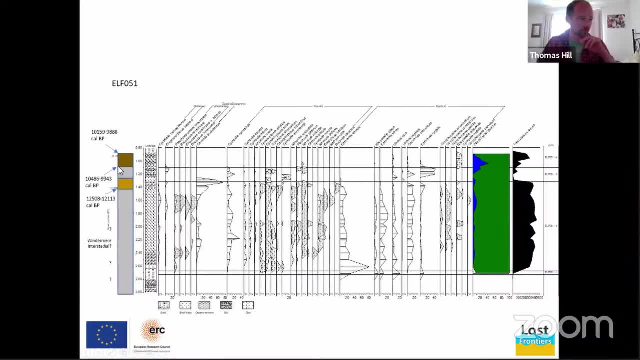 and in very brief summary strats, slight stratigraphic variations in organic content. we infer Windermere interstadial for the lowermost section in which the diatoms are most abundant. We now have some freshwater plankton. in low numbers freshwater plankton are present. 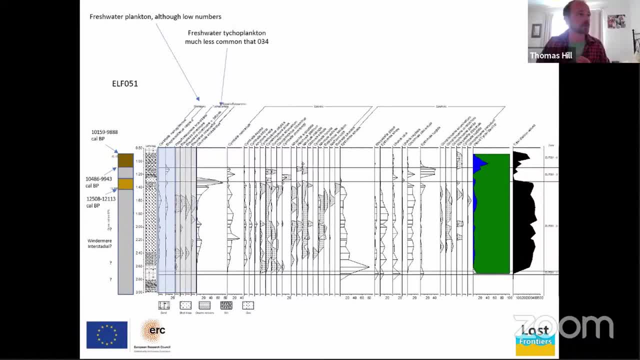 but consistent. we have a much lower presence of taika plankton. indeed, these little zones are being exaggerated because they're so low, so they're very small components. we're in this assumed Windermere, interstadial and vegetation thriving diatoms are much more. 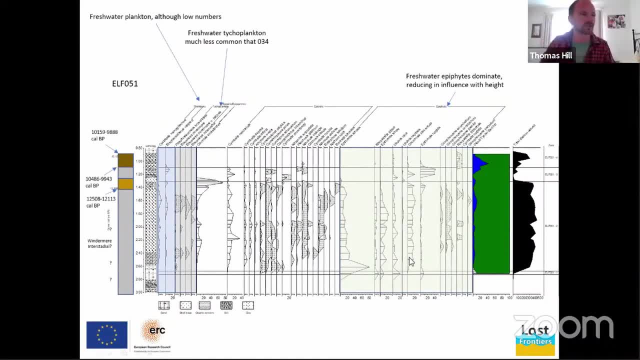 common. You can see the overall dominance we're looking at about 70%, 600mm, 60-70% of the diatom assemblage, with an overall decline in some of the key taxa with height towards this upper zone And in contrast we have a low but consistent number of epipellate taxa. 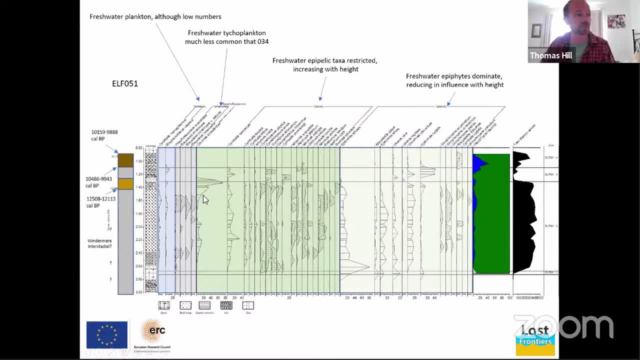 these are the muddy taxa, but there is an increase, quite a substantial increase, especially with one taxa called Cavanula scotoloides, which is a very cryptic one I found very little information about. However, it does increase quite substantially. prior to this, this is a zonal. 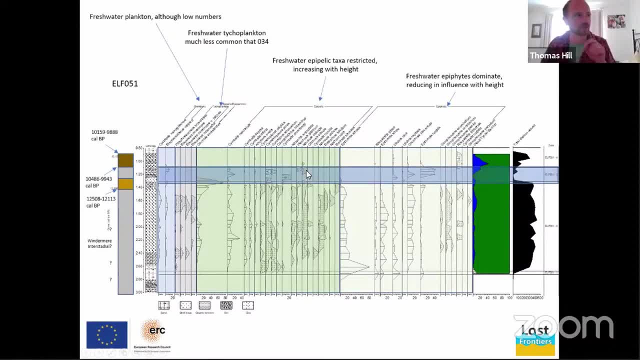 boundary that I've identified. This zonal boundary, however, is due to extremely poor preservation And if we take this all into account- poor preservation, the radiocarbon dates and this increase in muddy or sand dwelling taxa- we could start thinking about what's going. 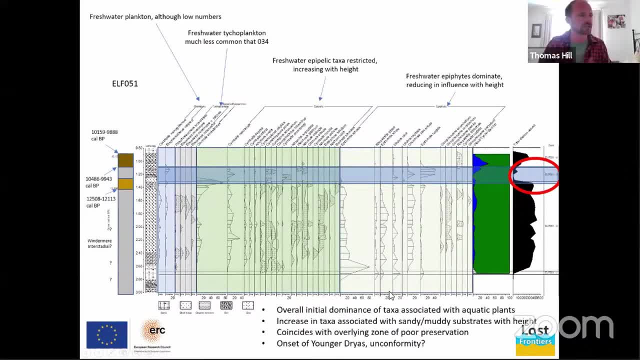 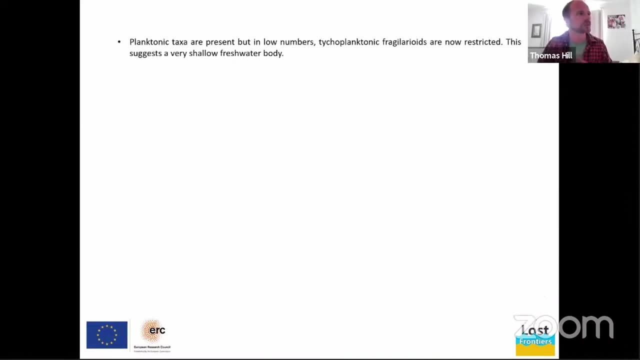 on Overall dominance of aquatics initially increased in taxa associated with sandy or muddy substrates coinciding with an overlying zone of poor preservation. Could this be an evidence of an unconformity? or indeed the younger dryas? So planktonic taxa are present in very low numbers. type of planktonic fragilarioids are: 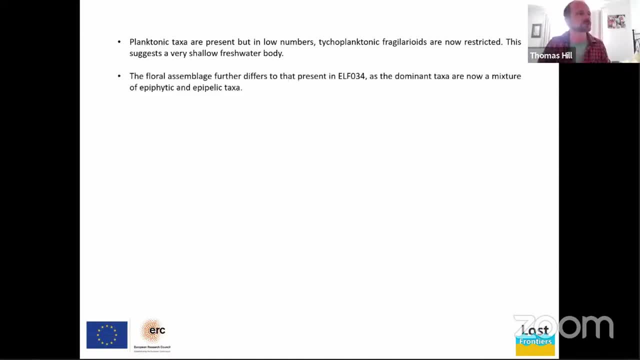 now restricted and it suggests a very shallow freshwater body. The floral assemblage further differs to 34, in that now epiphytes and epipellate taxa are dominated. The epiphytic taxa dominate. they dominate in the base but decrease in height over time to be replaced. 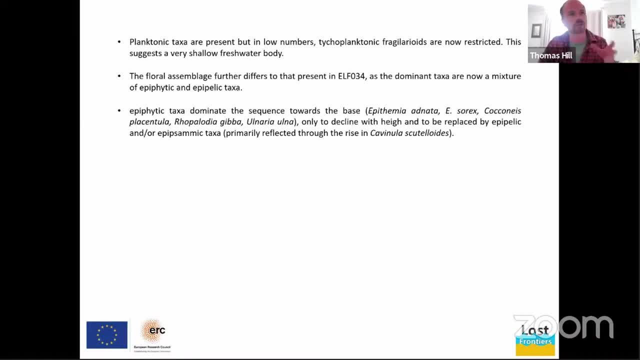 by this taxa Cavanula scutellides, which is associated with sandy and or muddy substrates, And if we can retain confidence, as we have with the radiocarbon dates, this then shifts into very, very poor preservation. with height, we could be looking at actually a climatic 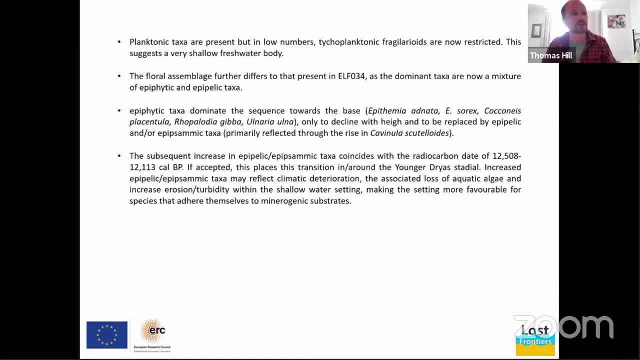 signal preserved within the diatoms as well. The transition in and around the younger dryas, resulting in increased epiphytic epiphytic. epiphytic tachsa is a result of climatic deterioration, associated loss of aquatic algae and the increase in erosion of subidium. 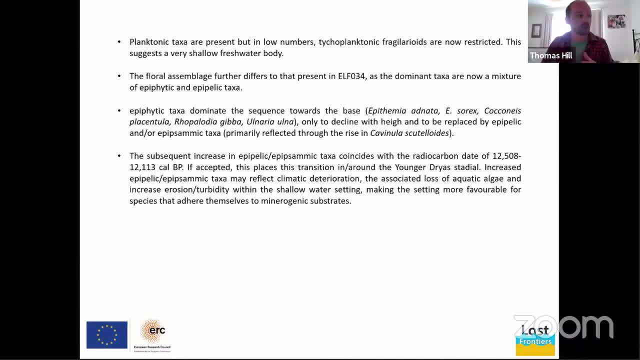 turbidity within a very shallow water setting, making the setting more favourable for species that adhere themselves to mineralogenics. And again, just to reinforce this, we then have this much more epiphyte rich sequence underneath to which, again, we're going to: 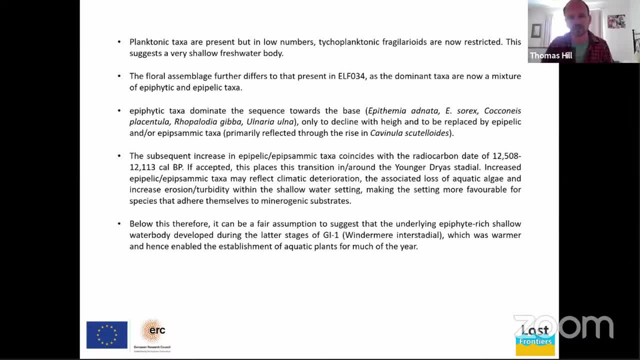 be working with the dating team to get a greater understanding of the age of this section, because at the moment we're reliant on a single AMS radiocarbon date to the top. I'm sure Tim will have information about these sequences as we continue on with regards to the OSL. 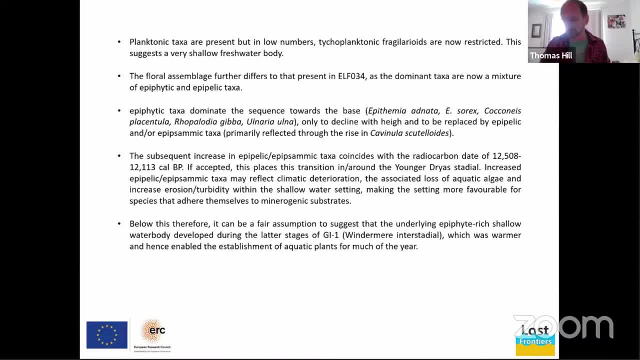 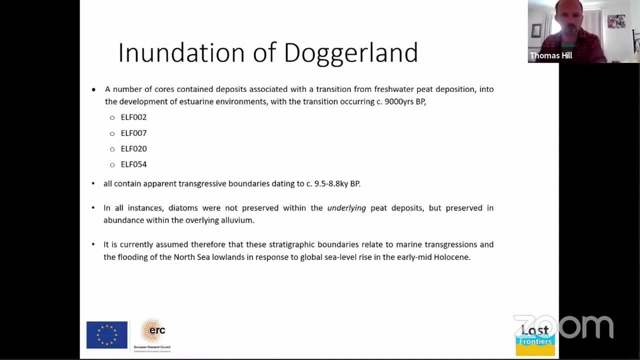 We can be confident that we're looking at the Windermere in Stadial, based on the abundance of epiphytes and an assumption that there is a lot of organic plants living in and around this setting. All right, five minutes to go. I think I'm doing all right. 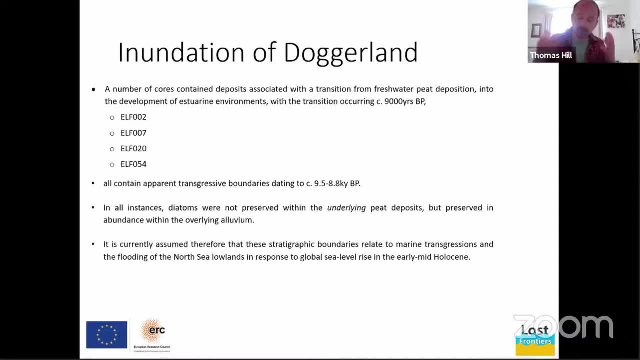 The second aspect, and just as significant, is obviously one of the key drivers and objectives of this project was to understand the inundation of Doggerlands. you know the timing and the extent and the rate, and so on and so forth. And one of the best ways of doing that is when we find 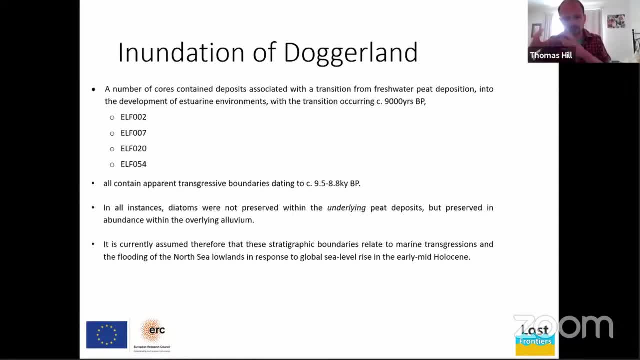 stratigraphic boundaries of clear freshwater into coastal deposition or estuarine deposition. Now, a number of the cores had a stratigraphic boundary preserved within, and I'll highlight a couple of them here. I'm only going to talk about one and then provide some general comments. 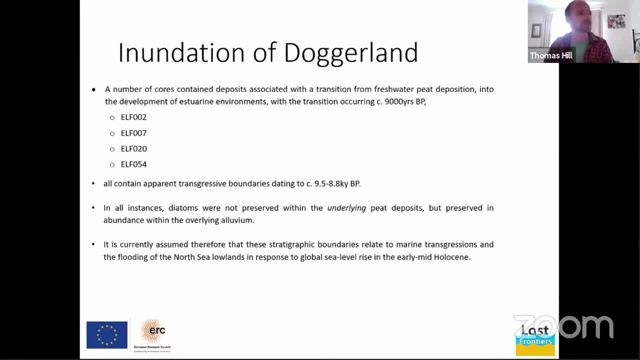 about the others as well, just due to time, But in general, all of them, all of these cores highlighted here, in which we have this freshwater peat to estuarine silty position, had a stratigraphic boundary dated to somewhere between 9.5 and 8.8.. And again, modelling will be done to understand. 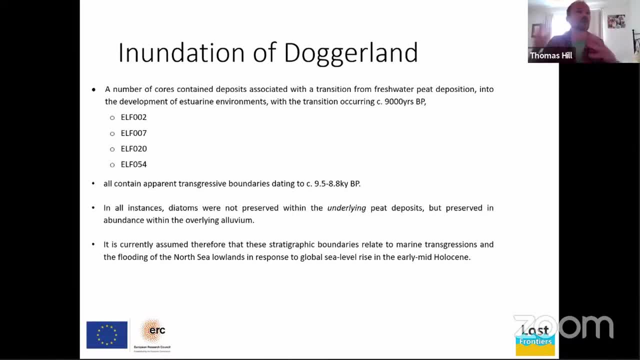 the extent and the accuracy and reliability of these things and what that tells us about the rate of change in due course. In all instances, diatoms were not preserved within the underlying peats. Now they do live in peatland settings, but the acids within the waters often dissolve the 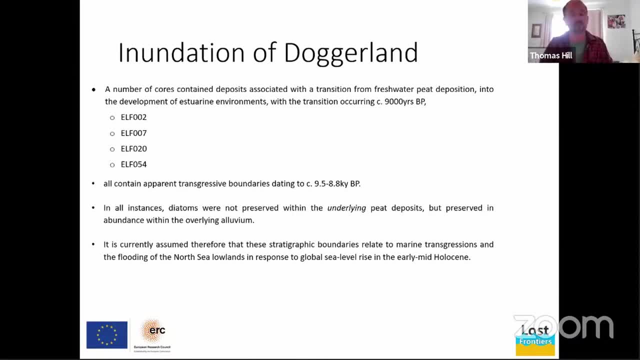 biogenic silica, So they're not always preserved very well in pure peats, but they were found in abundance in the overlying alluvium, And so therefore it's currently assumed that the stratigraphic boundaries relate to marine transgressions and the flooding of the North. 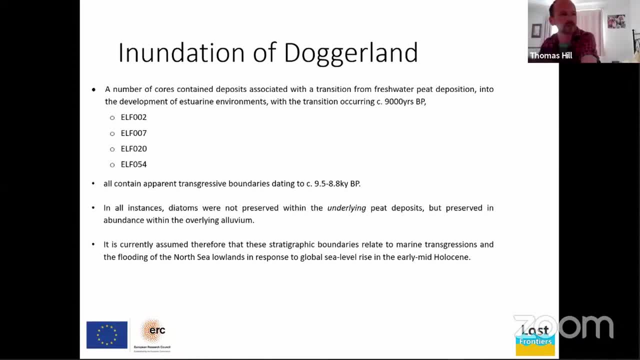 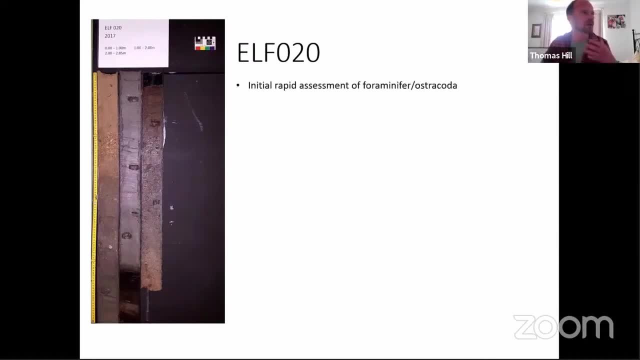 Sea lowlands in response to global sea level rise in the early Holocene. We've seen this beauty before. Ben alluded to it Again. John did initial rapid assessments and we did an initial radiocarbon dating. It's up to you if you'd like to take a look at that. And then, of course, there's a lot of 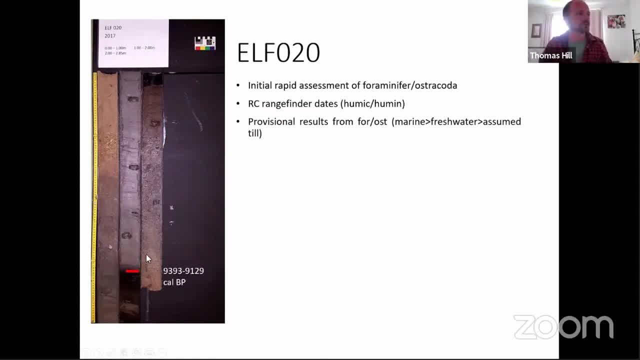 other things that we can look at, but I'm not going to go into too much detail here. I'm going to highlight that in ELF20, the transition from what was assumed till overlaid by freshwater deposition inferred by the microfossil work and then overlaid by these marine estuarine deposits- 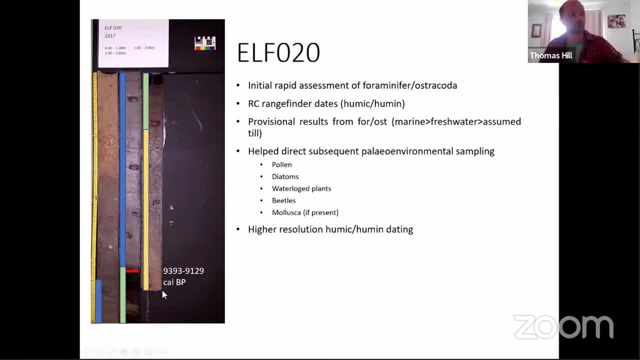 And this then directed, as it did with every core, further, fuller analysis, where preservation was found to be good And diatoms were found in abundance within the overlying strata but not within the freshwater peat. And here we have a very typical diagram of that boundary. 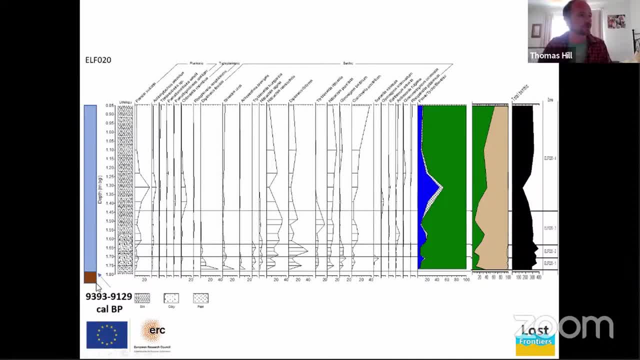 We have the radiocarbon date Here, we have the peat at the bottom, Diatoms are preserved And we have the alluvium overlying it And this is a very generalised summary of the diatoms that were encountered. We have a low but consistent presence of marine plankton. These attacks are 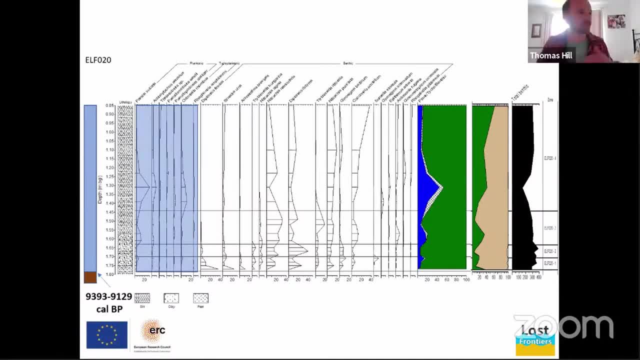 typical of open marine waters and they are present throughout And in general. this is a very typical indicator of the influence of tides and so on and so forth. But they are low, low and consistent, not majorly significantly contributing. The majority are benthic taxa And indeed throughout. 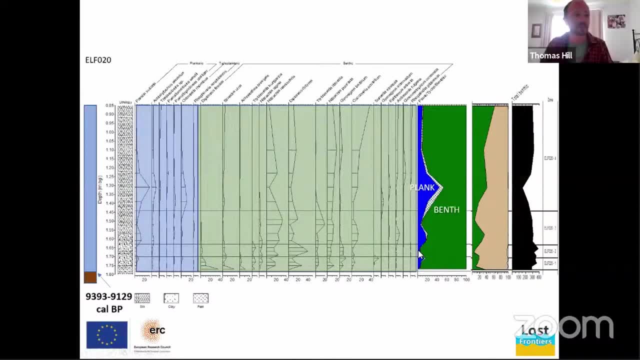 many of these cores, it was more often than not the benthic taxa dominated and the plankton were quite restricted in their preservation In a number of the cores. I think this is of interest in terms of understanding the landscape and the changing that took place Many of the cores have 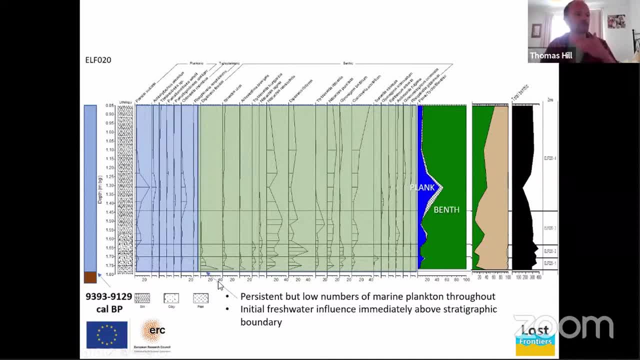 a few taxa that are, in relative abundance, immediately above the stratigraphic boundary, And these taxa are associated with much lower salinity conditions. In this instance, we're looking at Diplonose finica. In another core it was Navicular virigula. There are certain 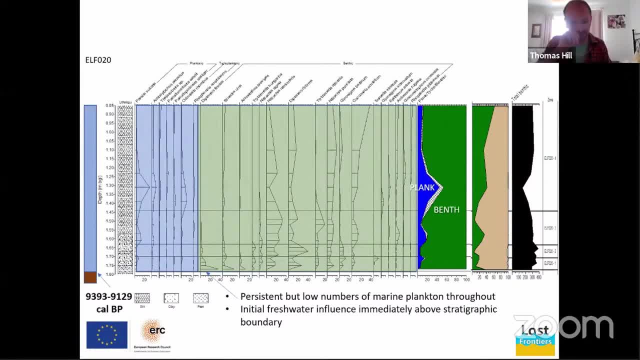 species that are much more associated with lower salinity conditions, encountered in abundance at the stratigraphic boundary and then reducing in height, to be replaced by the more typical marine brackish epipellate taxa, those attached to the body, substrates and epiphytes. 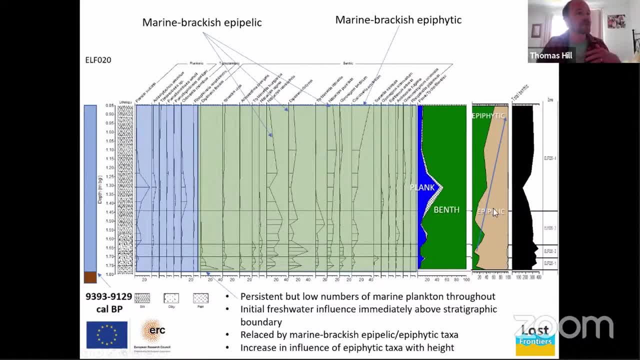 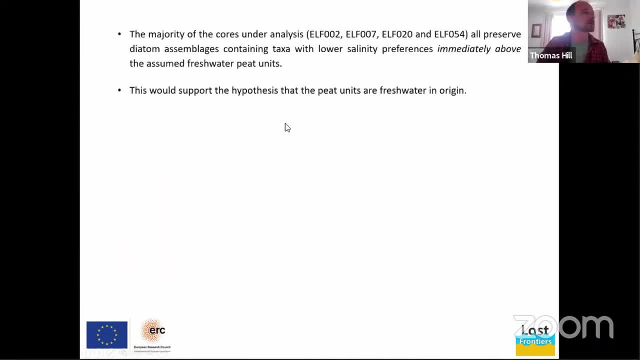 Oh, I'm going to have to run now, Okay. And then, in this instance, there's an increase in epiphytated taxa with height. Is it working? There we go. So to generalize the majority of the cores under analysis, all preserved diatom assemblages containing taxa with lower salinity. 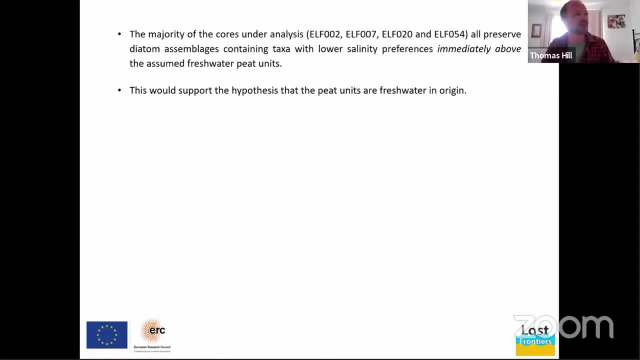 preferences immediately above the assumed freshwater units, And this would support the hypothesis, obviously, that the peat units are freshwater in origin rather than being a small peat body accumulating in an abandoned tidal channel or something similar on the mudflats. These boundaries are therefore all gradual and also unlikely to be erosive. This is one of the 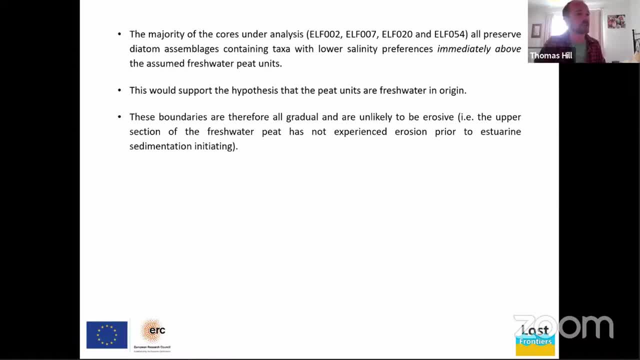 things I think is very important in understanding the role of relative sea level change, because potentially you could have a section of the peat being removed prior to the marine deposits accumulating, But the fact that we have these low salinity species immediately overlying would suggest that we're looking at a gradual, however you want to. 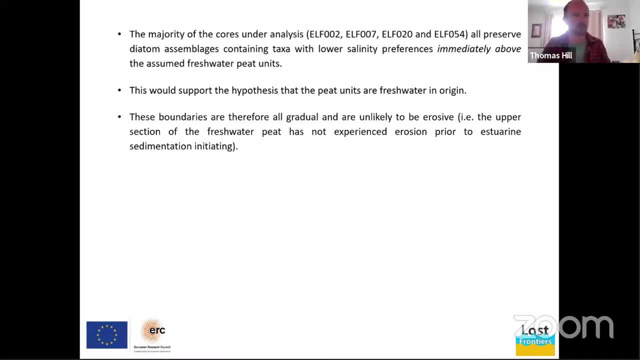 define gradual in terms of time scales, but a conformable shifting climate And in general the floral assemblages are dominated by either epiphytic or epiphelic and there is an overall absence of these taxa in the aerophilus ray, an epiphasamic taxa and generally restricted marine. 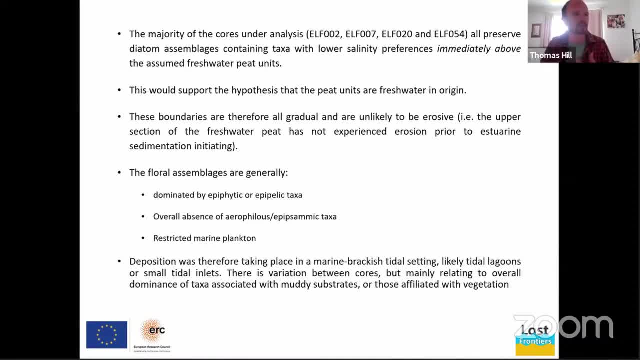 plankton And based on this, we think we're looking at marine brackish tidal settings, likely tidal lagoons or small tidal lagoons, And the fact that there's a general sense of a gradual shift in the climate and there's a general sense of a gradual shift in the climate and there's a general sense of a general 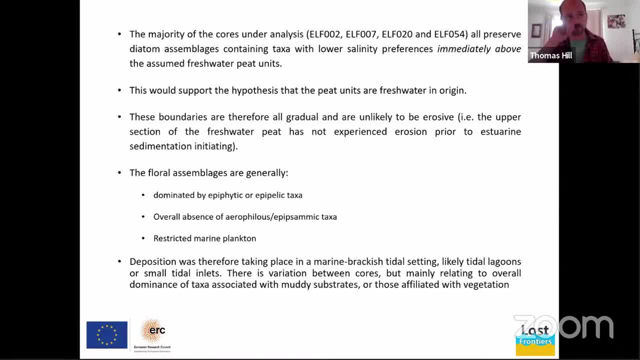 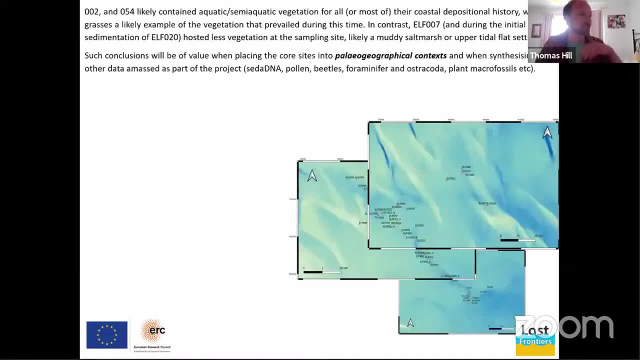 inlets rather than a very open coastline to account for these sort of assemblages being present. and just a final slide is just in terms of: we are very early in this assessment, in this analysis and interpretation. you know we have variations between these cores. so, for example, 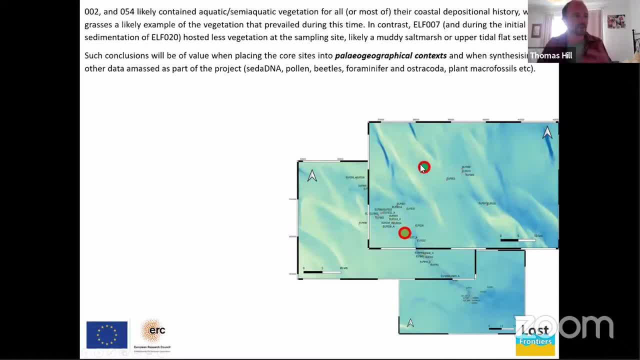 two of 54 are dominated by the epiphytes, to suggest a more of a vegetated coastal lowland, things like seagrasses, whereas some of the other cores are more the muddy substrates and and this will start helping us when we start putting them into paleogeographical context. 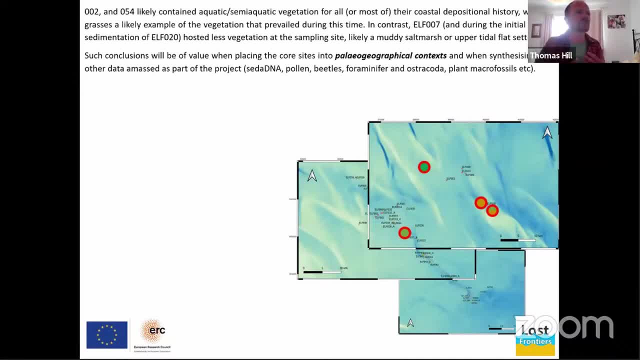 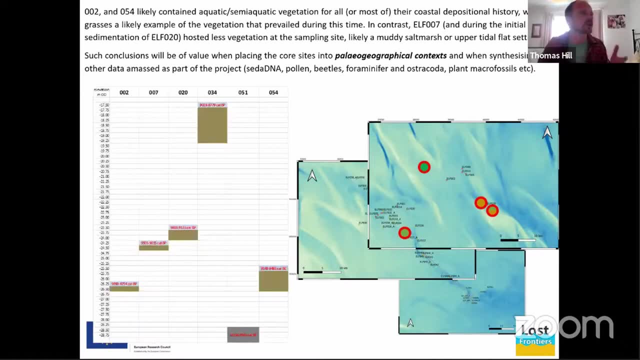 and synthesizing with the other data. you know i don't think we've got this lovely uniform shift from freshwater to marine conditions as sea level rise and this is highlighted by simply just trying to plot vertically the transition from freshwater peat into estuarine alluvium. the elevations don't. 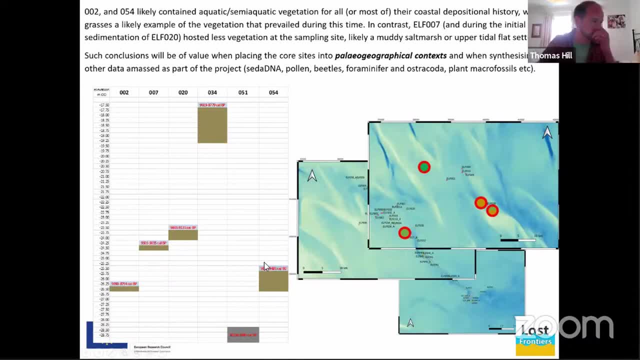 necessarily link to um, to the timings of the um, the transitions. some of the cores um, some of the cores that um were flooded latest by marine conditions, are um, were are some of the deepest cores. so, as highlighted by martin, we've got a really complex um geomorphological um picture to develop. first are we looking at: 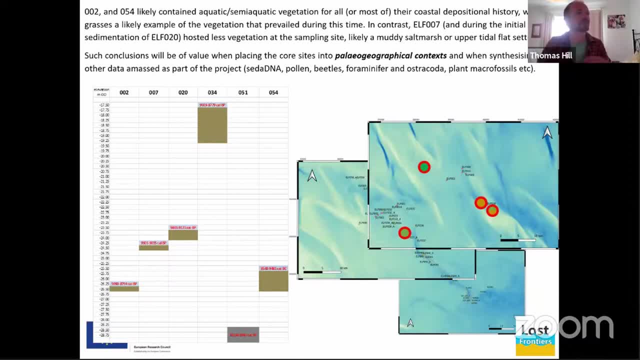 little isolation basins? are we looking at more of an open setting? you know what are the crustal movements to account for these vertical variations and so on. so there's a lot of things to think about and we are at the start of really starting to really synthesize this data together, but it's 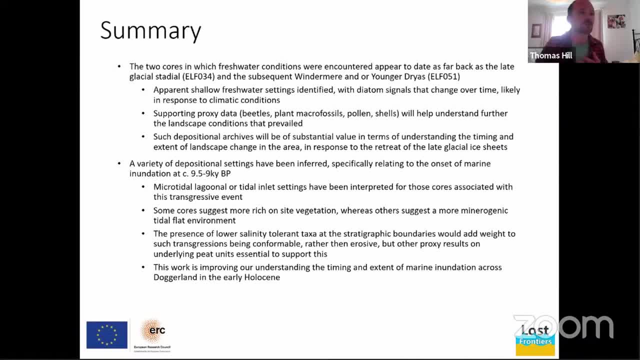 exciting. nonetheless, and in light of um richard being in front of me in the screen, i'm going to leave some of the summary um points up, um for and ask for any questions. thanks, tom, that's, that's really great. um, yeah, so just before questions come in, uh, david smith has